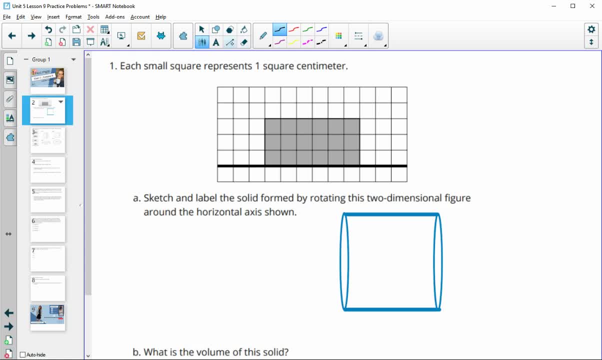 And then we've got the radius in here, So let me get that in a different color, But we've got the radius here at three, All right. so then it wants to know the volume of this. So remember, the volume formula is the area of the base times the height, And so we can find the area of the. 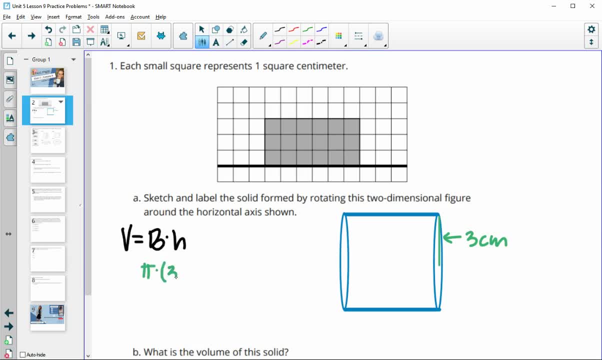 base by doing pi times the radius squared, since it's a circle. So that's going to be the area of our base, And then the height is going to be the distance between the bases, so from here to here, And so we'll just count how long this is, and that'll be the same. 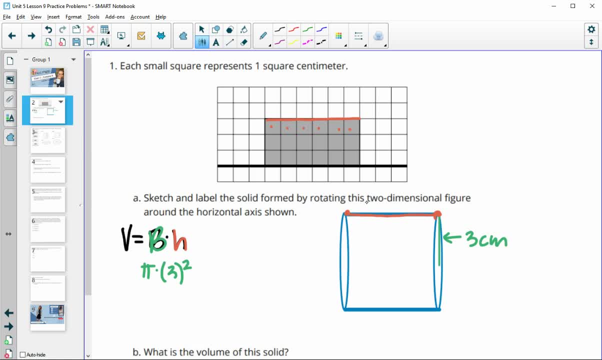 here. So this is one, two, three, four, five, six centimeters, And so then we'll multiply by six for that height, And so when you write out the volume, you can certainly do the decimal version. I'm just going to do three squared. 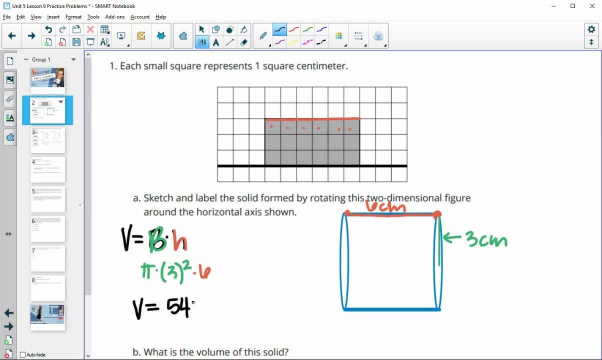 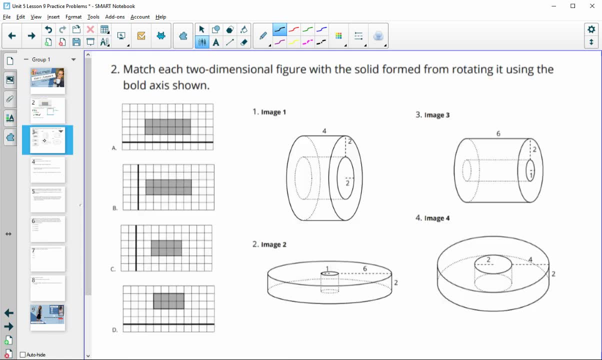 which is nine times six, which is 54.. So then I'll have 54 pi centimeters cubed for that volume. Number two has us matching the pictures with the two-dimensional figure, And so you can kind of narrow some of these down. So this one, we're rotating around a horizontal. So our hole. 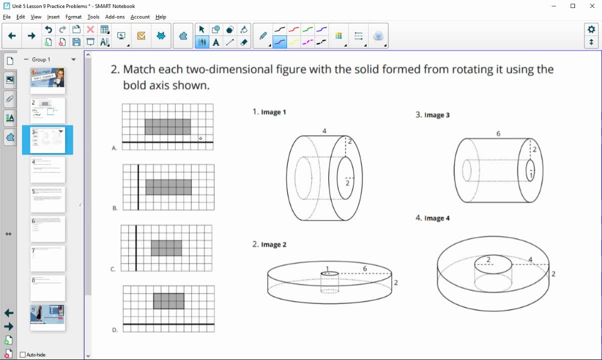 is going to be going horizontally when we're rotating vertically like this. So a picture that would match with a horizontal axis of rotation would be so A and D, they would match. So this image is either A or D because it's horizontal, And image three is also A or D, So you can start to kind of narrow. 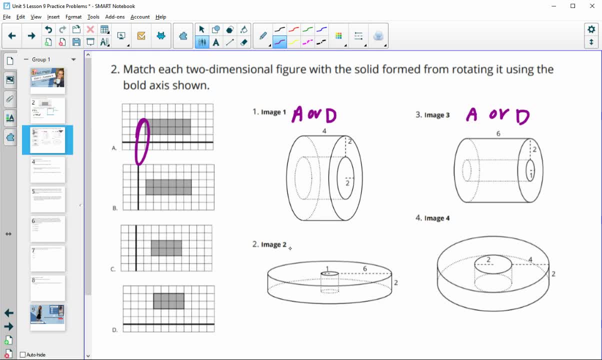 some things down. Then if we're rotating vertically, that's going to be these two, images B and C, And those go with image two or four. So then you're kind of just narrowing your, your options down here. So for this one A, this is going to have a hole that's one wide. 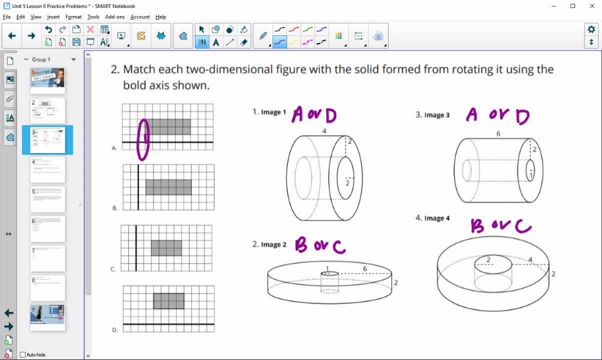 and then. so there's going to be a hole in there that has a radius of one And then kind of the width after that is going to be two. So if we take a look at this, this one, this one has the hole with a radius of one. 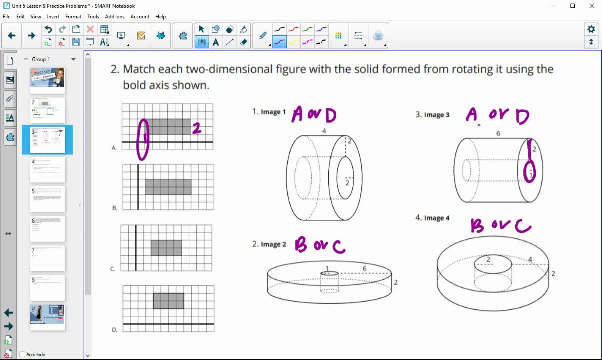 And then the width of kind of that disc is a 2. And so we know that this is image A. So then that leaves this one as image D And we can make sure. so it's got. you know, the inner part here would have a radius of 2.. 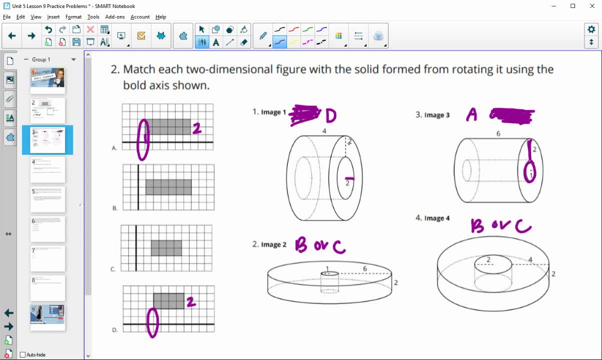 And so with this outer part. so we see that the inner radius is 2 and this disc radius is 2.. You can also see the different lengths here, like this one is, the height is 4.. So that matches. And this one, the height is 6, which matches. 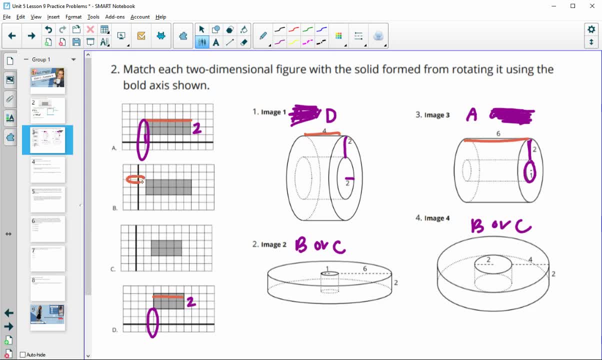 All right, then, to match these other ones. Now, when this one rotates around again, it's going to have a radius of 1 in that center hole, And so that would be this one, And so then that leaves C for this one, which we can see does have a radius of 2 for that inner part. 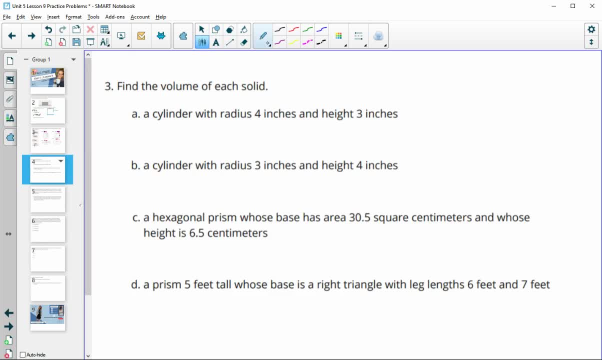 Number 3, find the volume of each solid. And so if we look at the different types of solids here, we've got a cylinder, we've got a cylinder, we've got a prism and then we've got a prism. So the volume formulas for each of these are going to be the area of the base times, the height. 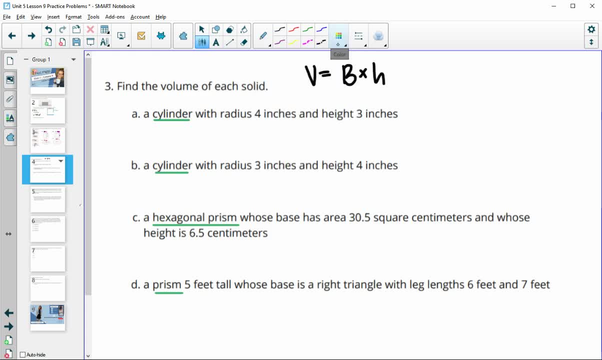 So we're going to have to find the area of each base, And so in this first one we've got a cylinder, So the base shape is So we'll be doing pi? r squared for that, So the radius is 4.. 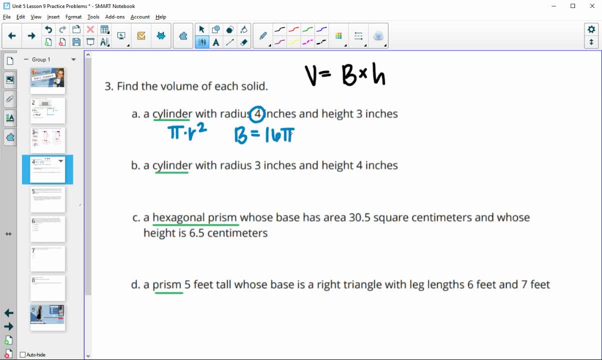 4 squared is 16 times pi. So there's the base area, And then we have the height of 3.. So the volume is going to be 16 pi times 3, which is 48 pi, And then inches cubed. 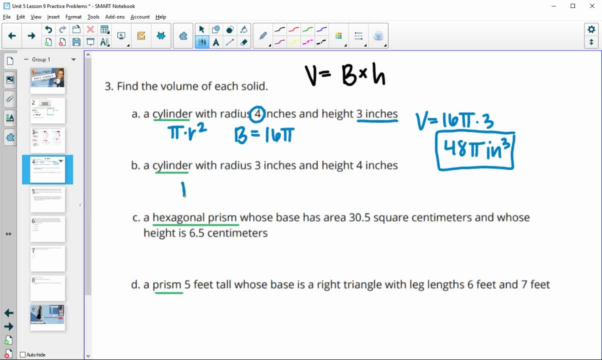 We have another cylinder in this next one, So we're also going to be. We're doing pi times the radius squared, And so the radius in this case is 3.. 3 squared is 9.. So the base area is 9 pi. 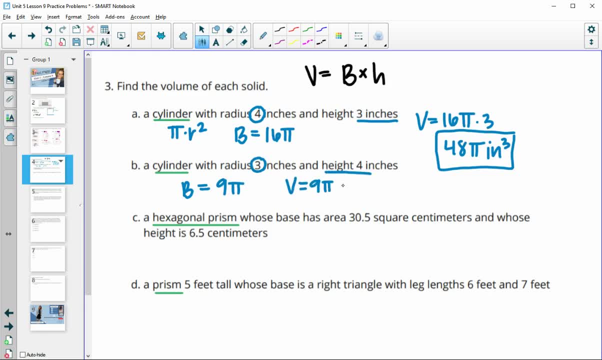 And then we'll be taking that base area times the height of 4.. So the volume here is going to be 36 pi inches cubed, And you could certainly multiply the pi in to get the full decimal. for this C gives us a hexagonal prism. 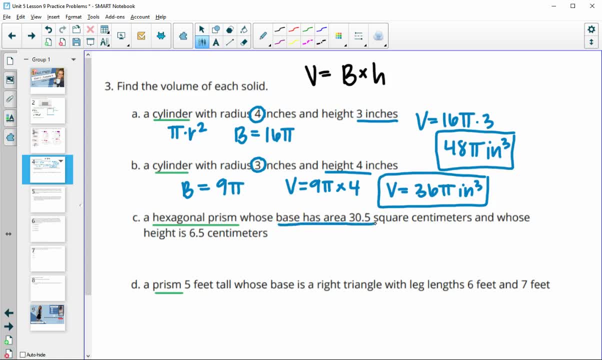 And then they tell us the base area. So we know the base area is already 30.5.. So we'll be doing 30.5 times the height, And then the height is 6.5.. So this is going to give us our volume area of the base times the height. 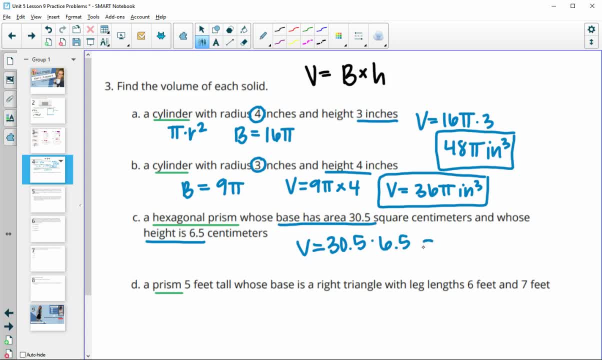 And 30.5 times 6.5 equals 198.24.. 5 inches cubed for that volume, Then we have a prism that is 5 feet tall. So here's our height, And then the base is a right triangle. 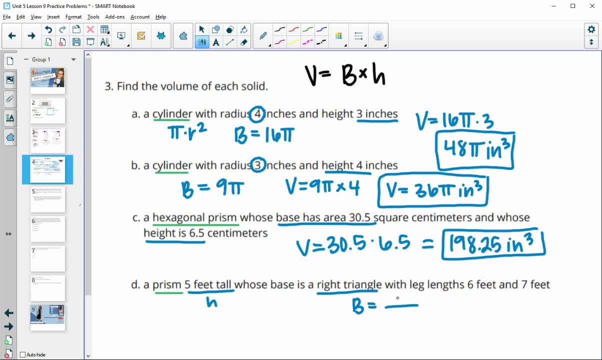 So, when we go to find the area of this, it's going to be the base times the height divided by 2. And so we have a right triangle. So we know, then, that the legs are the base and the height, And they're 6 and 7.. 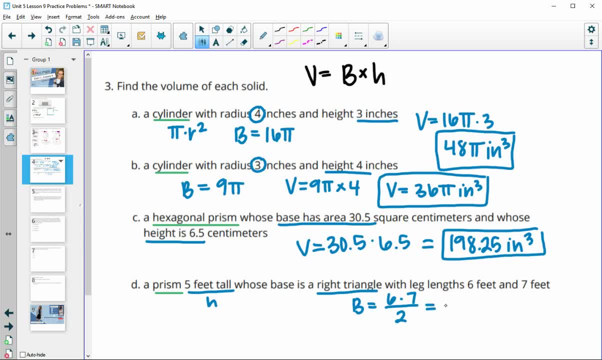 So we'll do 6 times 7,, which is 42, divided by 2,, which gives us 20.. 21 for our base area, And then we will take that times the height. So we will be doing 21,, which is our base area. 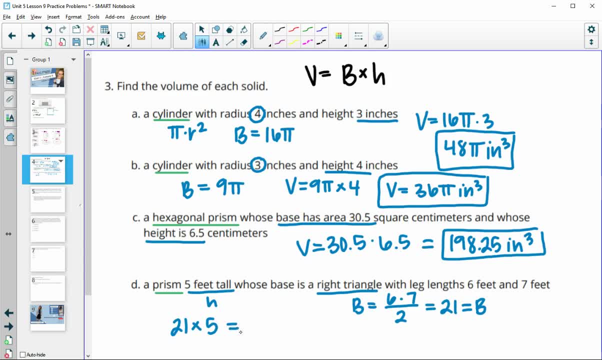 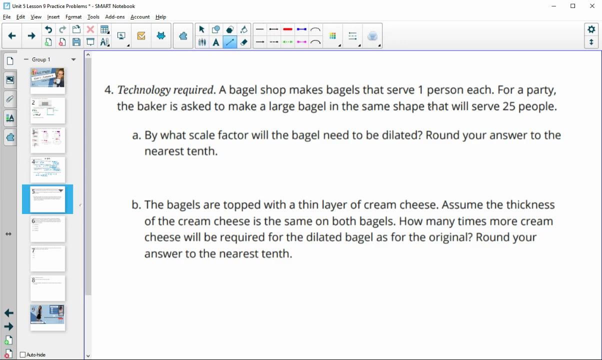 times 5, which is our height, And that will give us our volume of 105 feet cubed. Oh, and then this should be centimeters cubed, not inches, since they said centimeters there. Number four: a bagel shop makes bagels that serve one person. 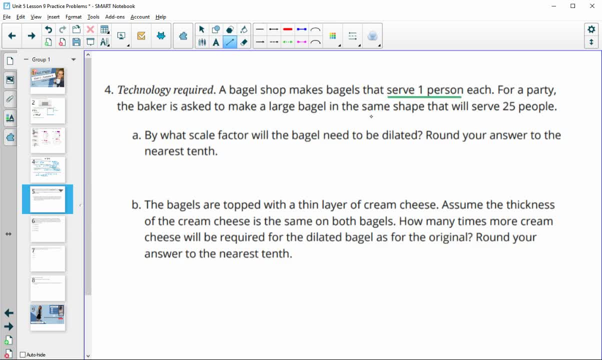 So they serve one person each. The baker is asked to make a large bagel, the same shape that will serve 25.. And people eat the entire bagel. So that's the volume. Okay, so they're eating. how much is being made up? 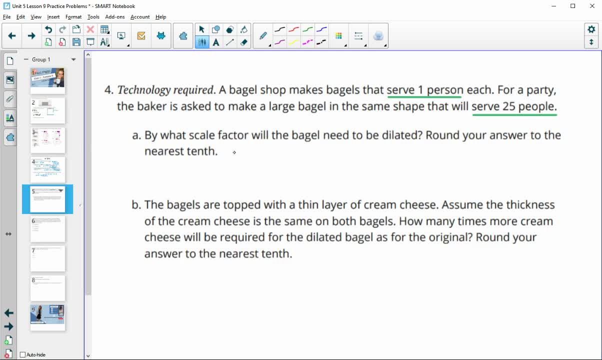 or how much is making up the bagel. So we know that we have volume when we compare the new to the old or the new to the original. So this is giving us our K cubed. So then we will cube, root this to figure out the actual scale factor here. 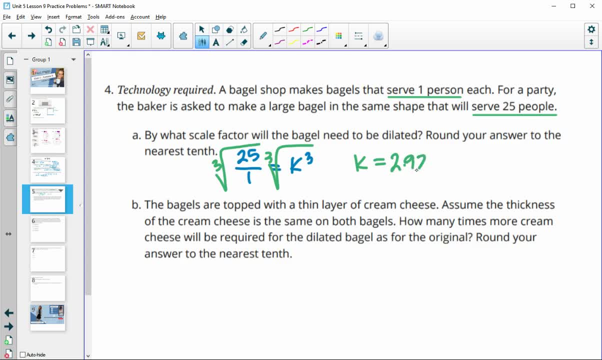 And when we cube root this we get 2.92.. Then in part B it asks us we're going to top the bagel with a thin layer of cream cheese. So this is going to be area. So how many times more cream cheese will be required? 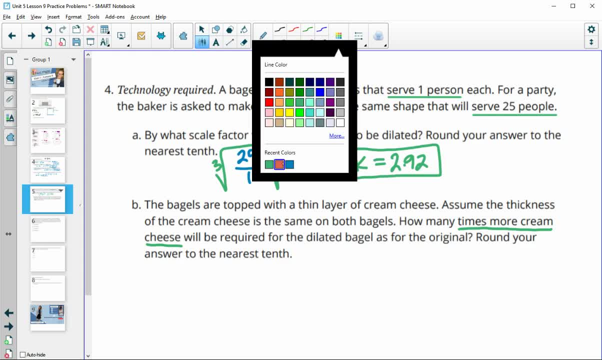 Um, if it's, if it's dilated from the original. So now when we're talking area, then we would want K squared times more. So we're going to be figuring out K squared, which is 2.92 squared. 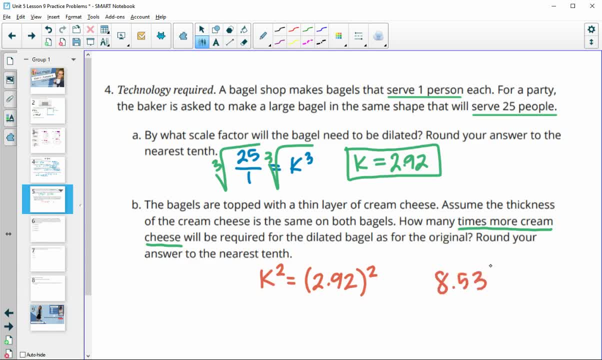 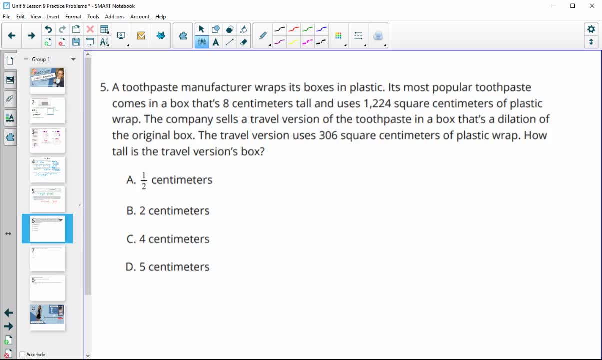 And so we are going to need 8.53 times more cream cheese. Number five: a toothpaste manufacturer wraps boxes in plastic, So wraps boxes in plastic means we're going to be dealing with area It's most popular. toothpaste comes in a box that's eight centimeters tall. 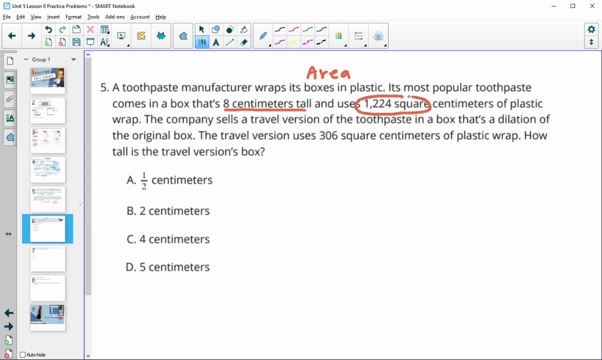 and uses 1,224 square centimeters. So here's the area. The company sells a travel version of the toothpaste in a box that's a dilation of the original. The travel size uses 306 square centimeters. How tall is the travel box? 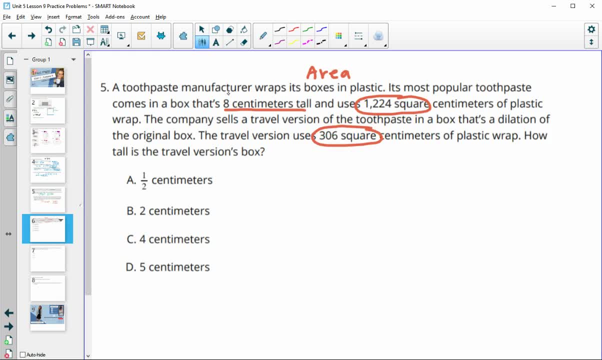 So we're going to need to come up with with the scale factor so we can use that on this height. So they gave us the new area and they gave us the original area. So we know we can figure out K squared this way. 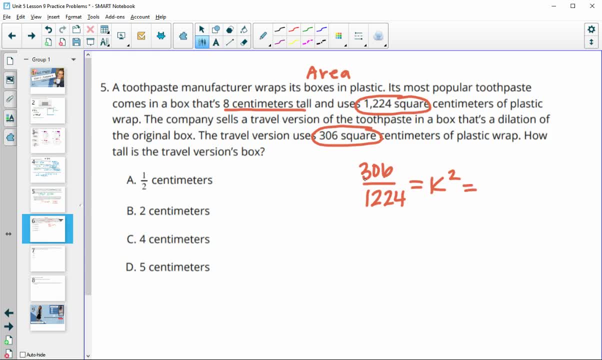 And so when we simplify that down um 306 divided by 1,224, that gives us 0.25, which is one fourth. So then to get the scale factor, we'll square root that. So our K value is 1.25.. 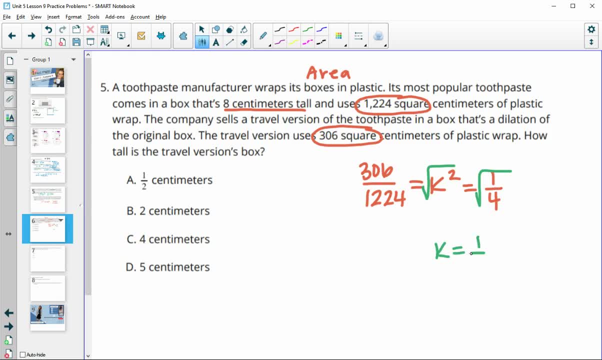 So then, to get the scale factor, we'll square root that, So our K value is equal to the square root of one, which is one, and the square root of four, which is two. So our scale factor is a half. So now we're going to take the original height. 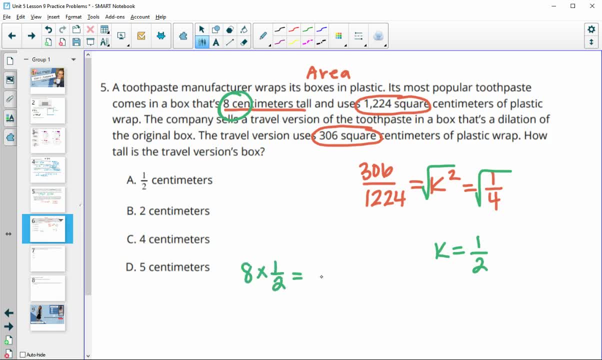 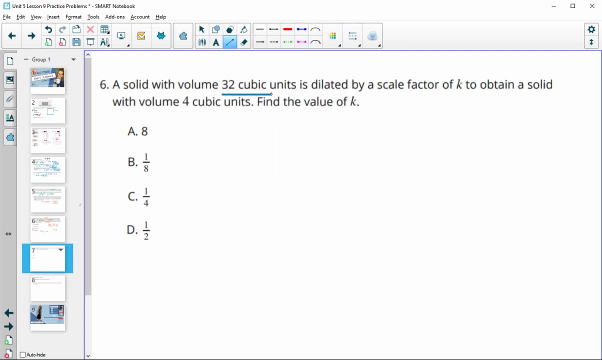 which is eight, and multiply it by the scale factor of one half And that will give us four centimeters. Number six: we have a solid with a volume of 32 cubic units. It's dilated by by a scale factor to get us four cubic units. 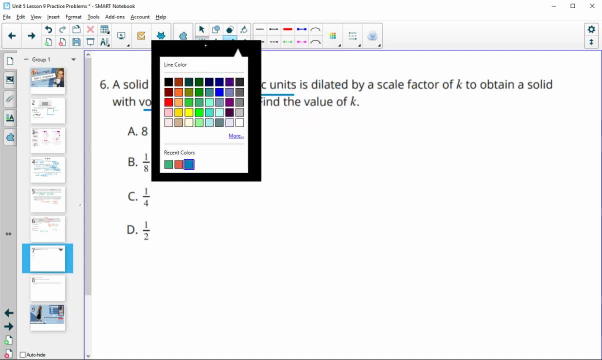 find the scale factor. So when we compare volumes, we remember that the new volume divided by the original volume is our K cubed value, and four over 32 simplifies to one eighth. So this is our K cubed. So then we will cube root this to figure out what our K value is. 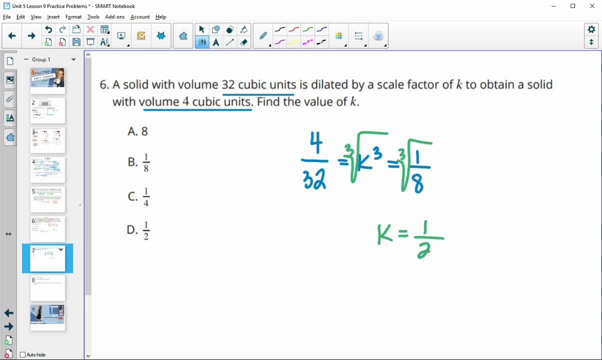 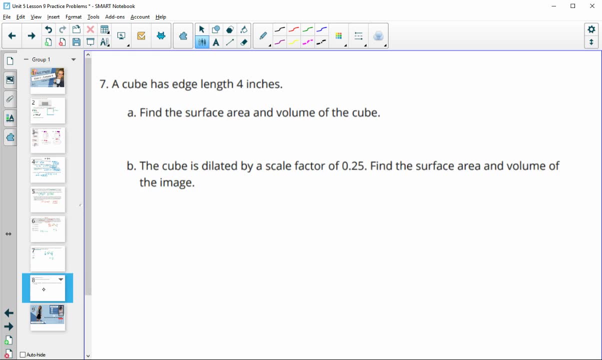 And the cube root of one is one. The cube root of eight is two, So the scale factor is one half, Then number seven. we have a cube that has edge lengths of four centimeters. find the surface area and the volume Um. 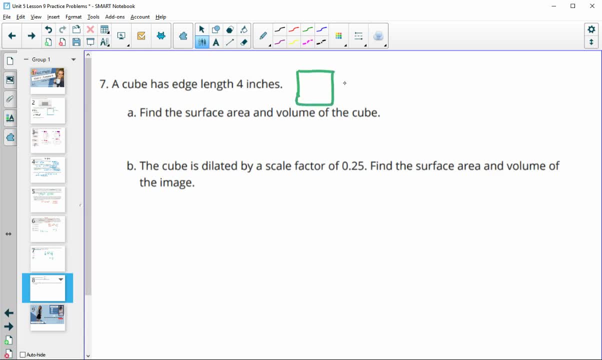 so we know that a cube has is made up of six squares, And so each of these are four by four squares, So the area of each square is 16.. So our overall surface area is going to be the area of one square times six. 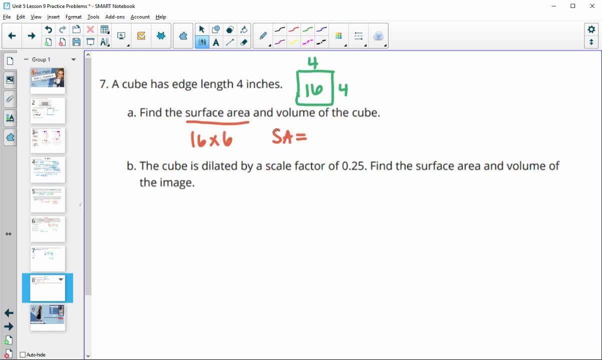 since there are six of them. So the surface area here is going to be 256 inches squared, And then the volume is going to take the area of the base, which is 16, and multiply that by the height And we know the height. 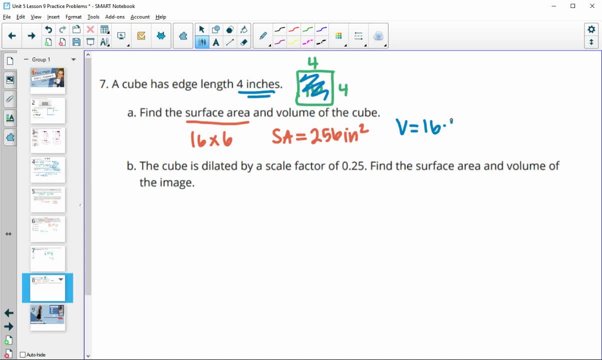 which would be the same length of this square, So times four. So if you think of, this is what a cube looks like. So we know that this base area is 16, and then the height is also four, So then the volume is going to be 16 times four. 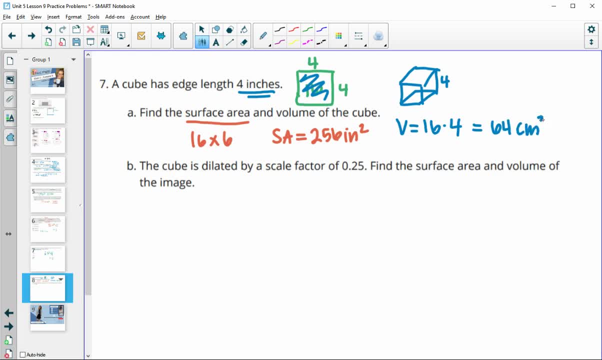 which gives us 64 centimeters cubed for that volume. Now the next part asks us: if we dilate these by a scale factor of 0.25, what will the new surface area and volume be? So if we take the original surface area and we multiply it by the scale factor squared, 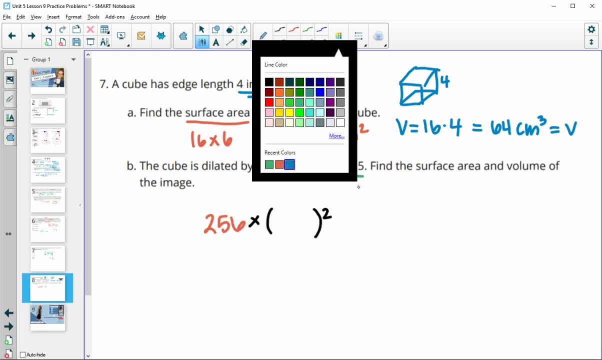 we'll have the new surface area And if we take the original volume and we multiply it by the scale factor cubed, we'll have the new volume. So 256 times 0.25 squared And then 64 times 0.25 cubed will get us our new answers.